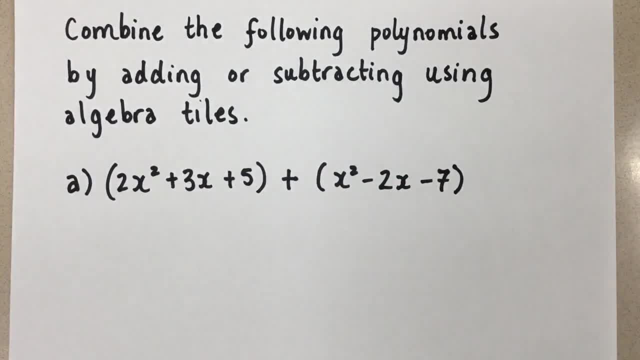 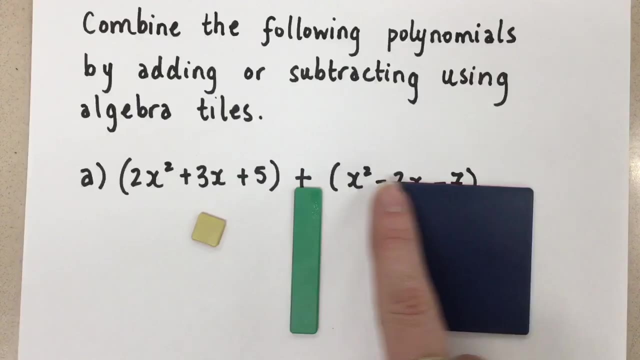 ourselves of the algebra tile pieces. Let's start with this one. actually, This is a positive one. Then this one's going to represent x- assuming we don't know the length of it, so we'll call it x. And then this one will represent x squared, because we have x times x gives us an x squared. 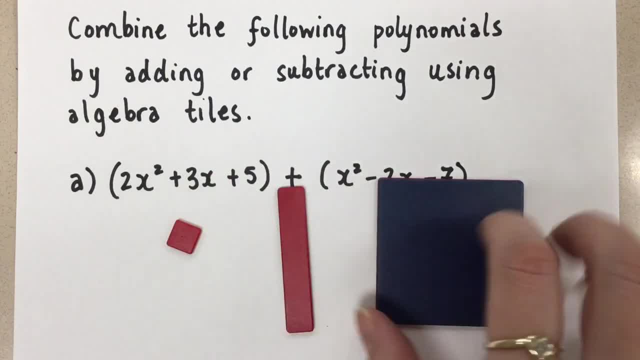 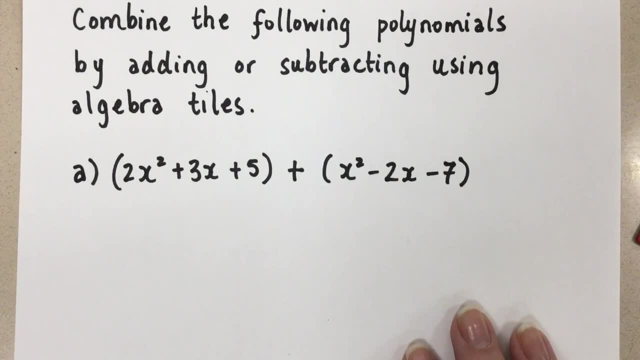 So those are the values. If we want them to be negative versions, we flip them over to see the red side and that would make them negative. So we want to begin by looking at the expression that we have. We have this polynomial plus this polynomial, So we're going to first 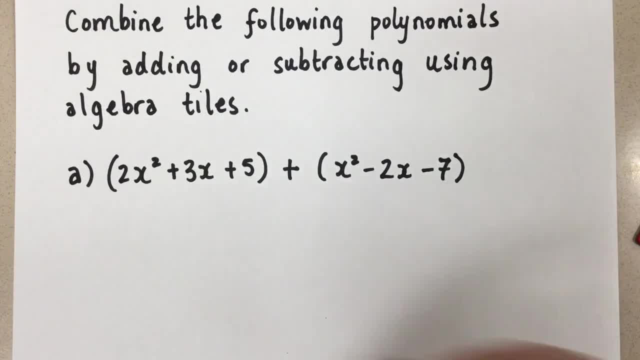 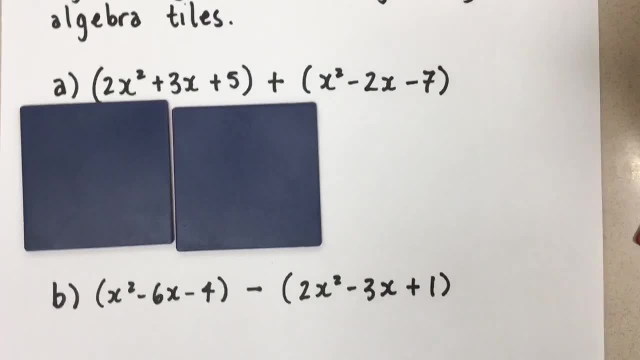 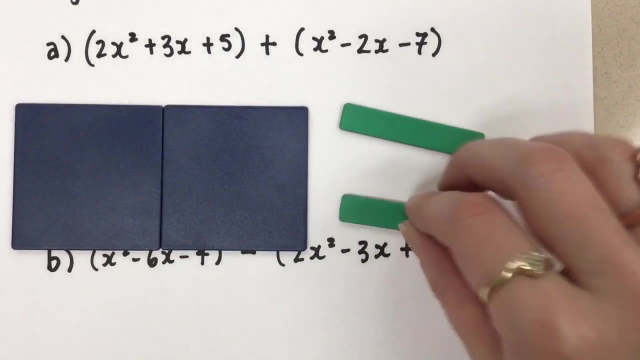 get the tiles that represent this polynomial here. So that is 2x squared, like this: Let's move this up a bit so we have some space: 2x squared and 3x. So this 3x is there and then five ones. 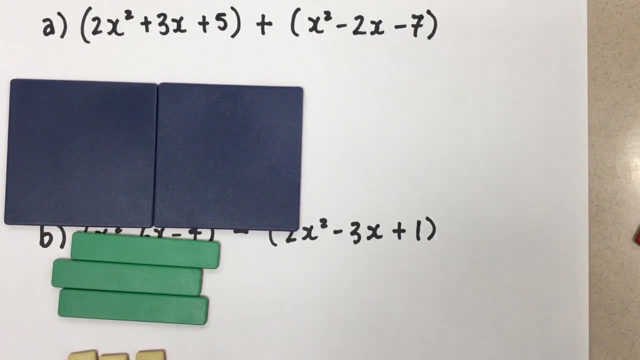 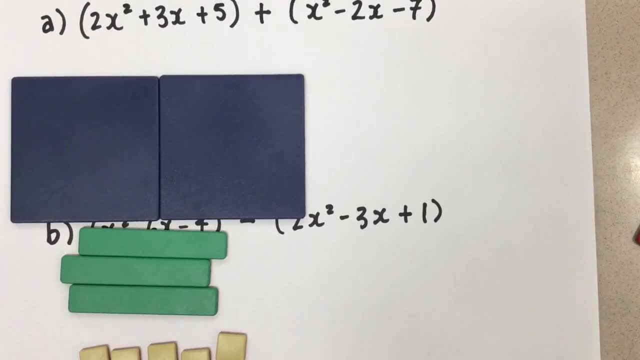 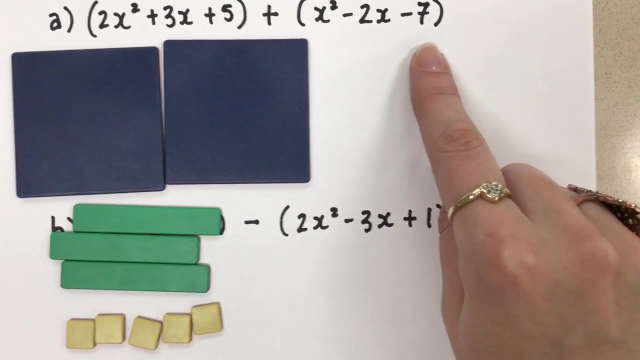 We want them to be positive: Three, four, five, Okay. so there we have 2x squared plus 3x plus five. Okay, now we want to get all of the algebra tiles that represent the second polynomial here, So the second polynomial, x squared minus 2x minus seven. So we'll start with an x squared. 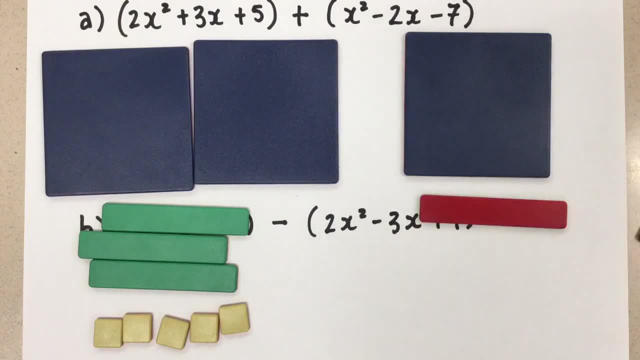 and then minus 2x. We need the red side of the x's, so there's minus 2x, And then we need minus 7.. So we need negative seven ones: 3,, 4,, 5,, 6,, 7.. 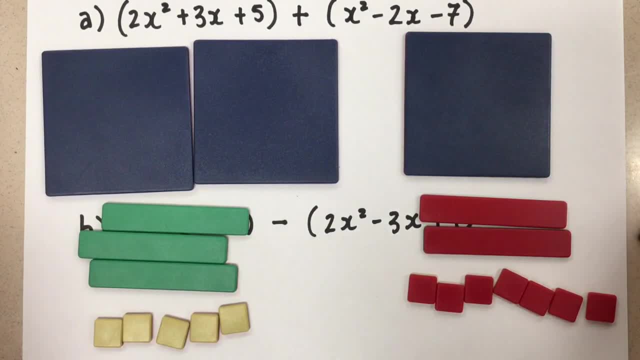 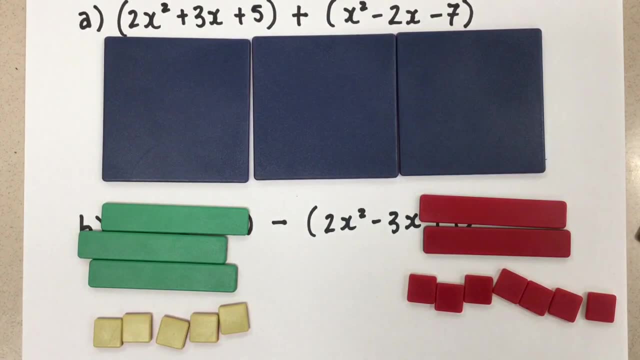 There we go. Okay, if we want to add these together, it's just a matter of combining these groups together. If we combine them together, what do we have? Well, we have 3x squared's. That's it. Now, with the x's it's a little more complicated. Let's look at this. 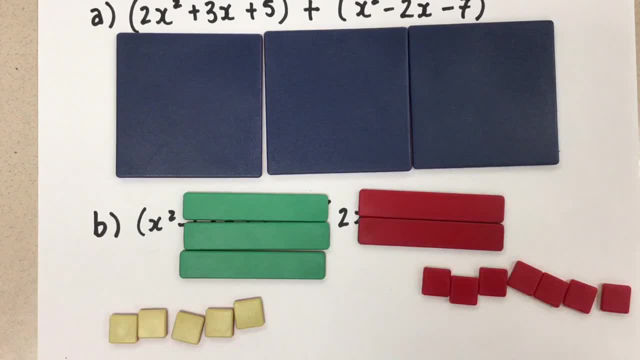 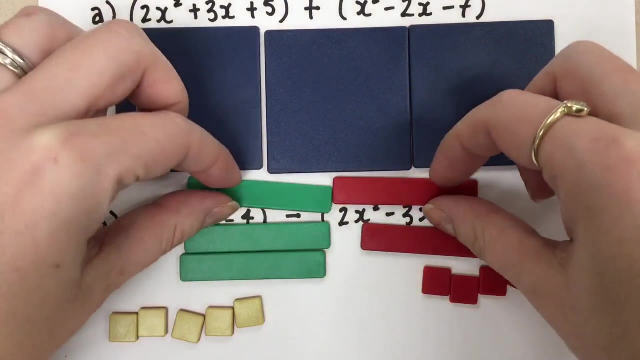 We have three positive x's and two negative x's, x's. So if we combine these together- a positive x and a negative x- that makes what we call a zero pair right. A positive x and a negative x added together is zero, So we can remove those That's. 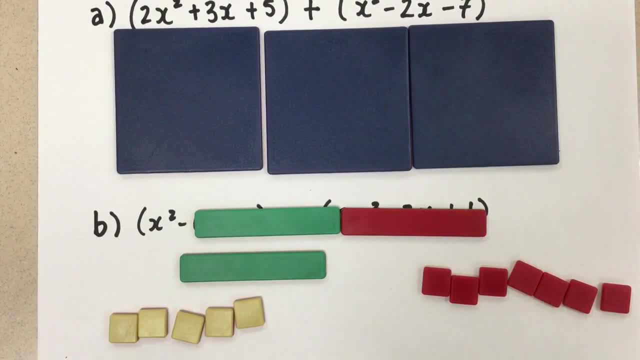 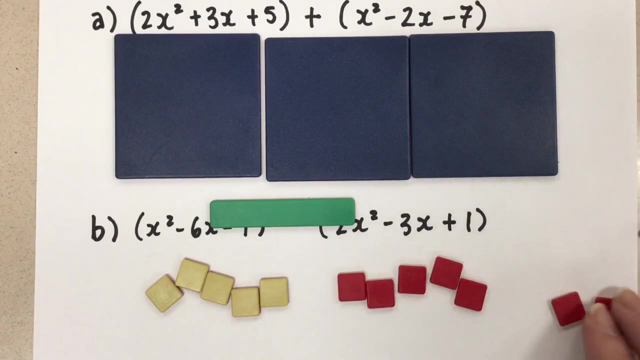 a zero pair, Let's get rid of it. And then we have another positive x and negative x. That's a zero pair again. We'll get rid of it And we're left with a remaining one x only, And then finally our ones. We had five positive ones and then we had seven negative ones. So if we do our zero, 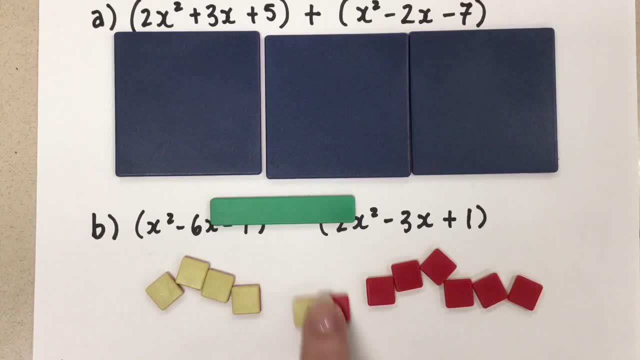 pairs again, a positive one and a negative one makes zero. Get rid of it. Positive one, negative one- zero. Positive one, negative one, another zero pair. Let's keep going. Positive one, negative one, zero pair. And finally a positive one and a negative one, another zero pair. And what are we? 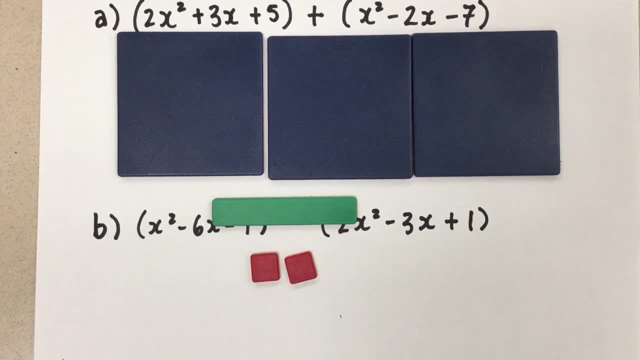 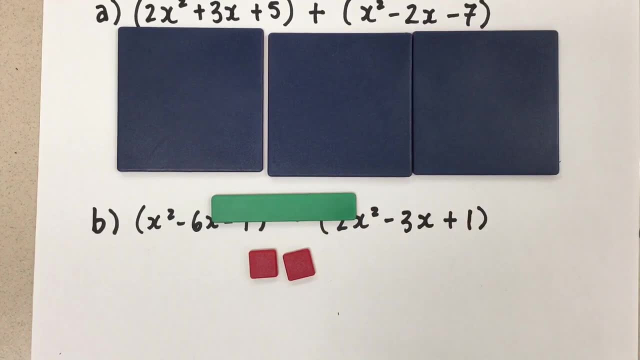 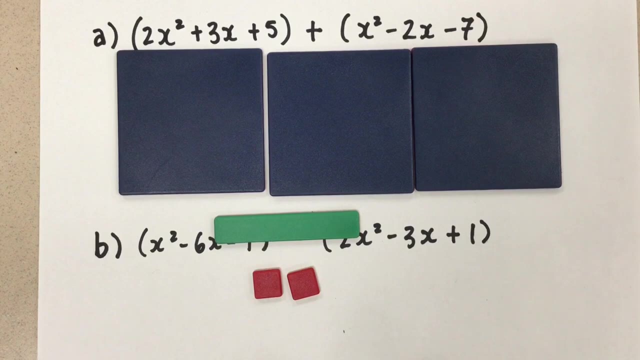 left with here Just negative two. So there's our final answer: Three x squared plus one x minus two. That's how we combine the polynomials using the algebra tiles. So now we have that visual of how these like terms are coming together. Notice how we only combine x squareds with x squareds. We only combine x's with x's. 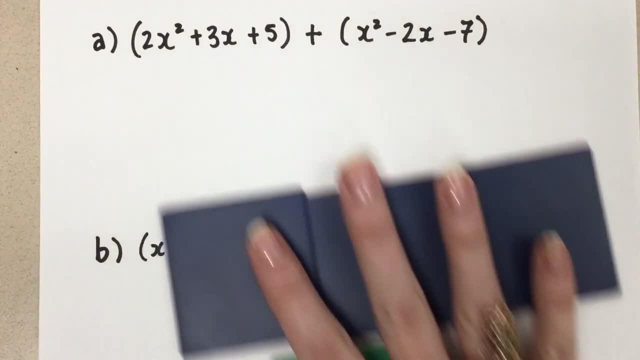 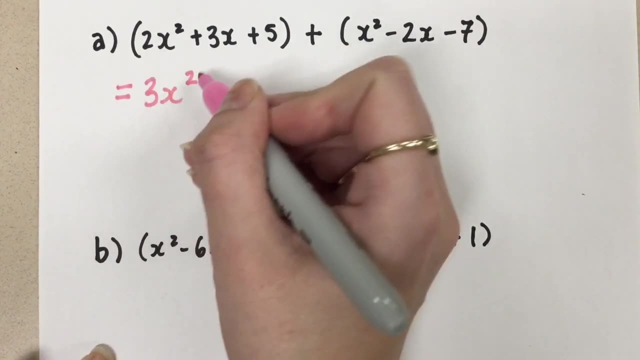 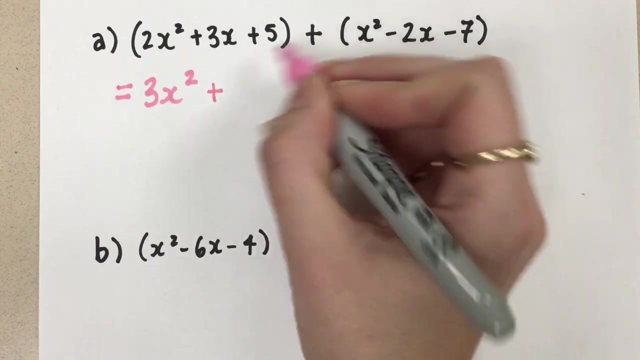 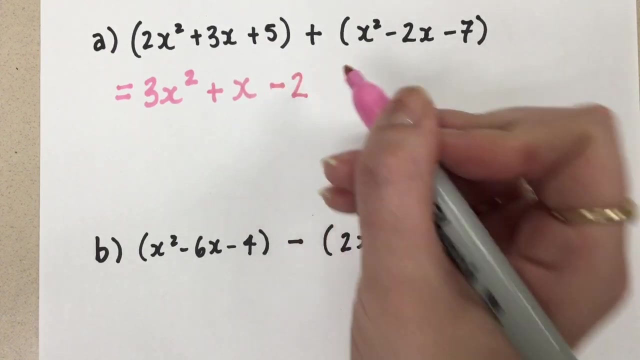 and we only combine ones with ones. Let's get our final answer written down here. So we had three x squareds And we had one x left. It was positive, And then we had minus two ones. So that is our final answer. 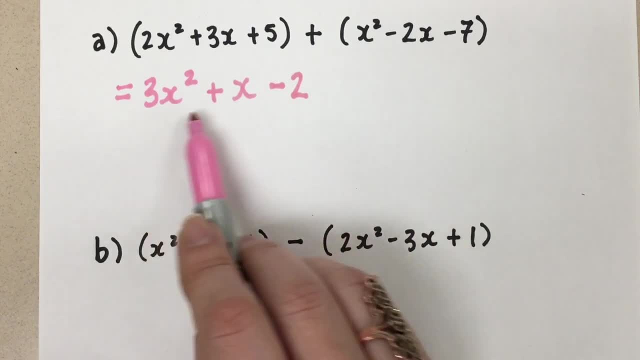 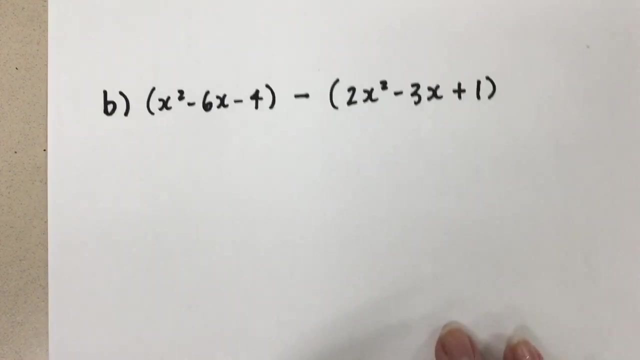 We do not want to combine these together because these are not like terms. They all have different visuals on the algebra tiles, So we leave it like that. That is simplified. Okay, let's try another one. We'll try subtracting polynomials now. So now we have this question: x squared minus. 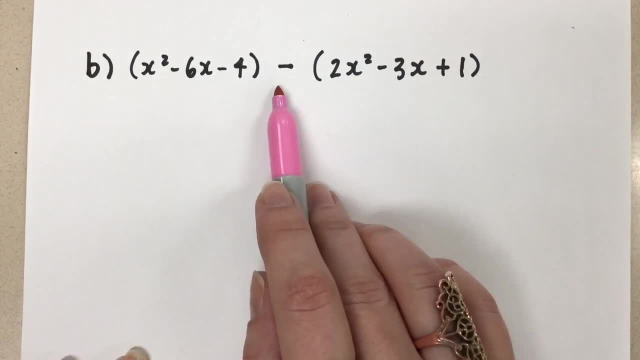 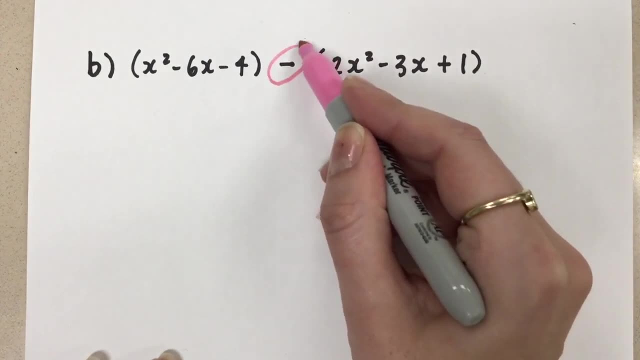 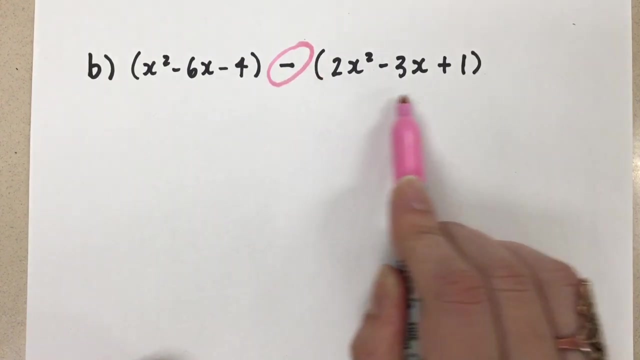 six x minus four minus two x squared minus three x plus one. So when we do this with that minus in between, now we have to make a little bit of a change. That minus there means that we're going to subtract this entire polynomial from this polynomial. 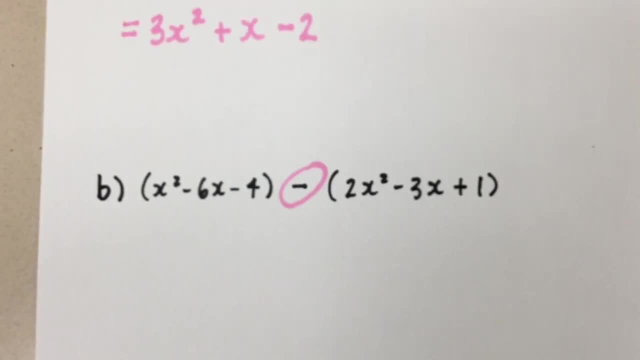 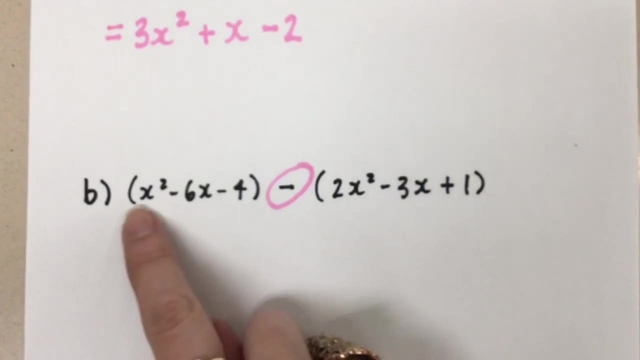 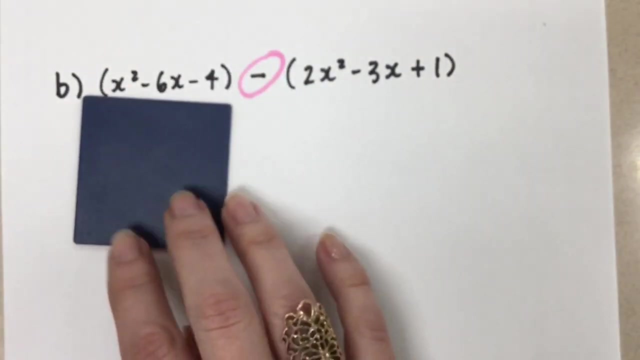 So we want to start this off in the same way that we would start the adding polynomials, like we did up here. So we're going to start by just getting the all the tiles that we need there for that first expression. So that is one x squared minus six x. 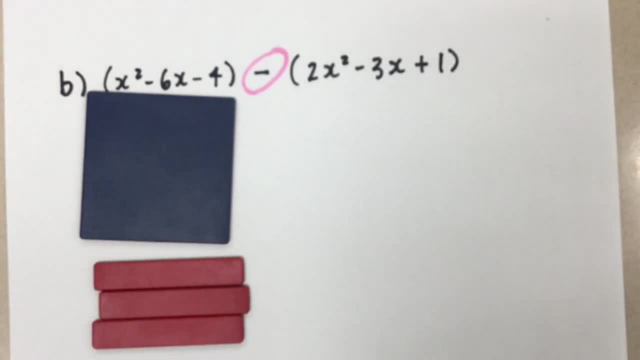 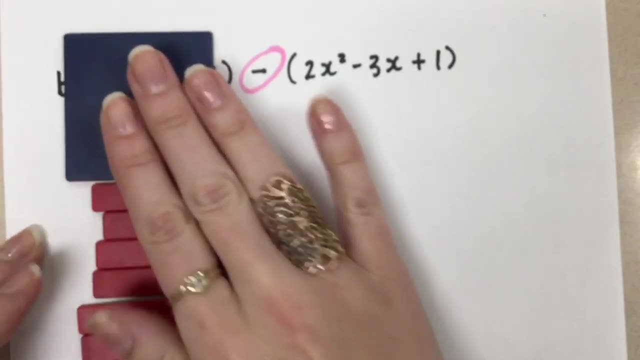 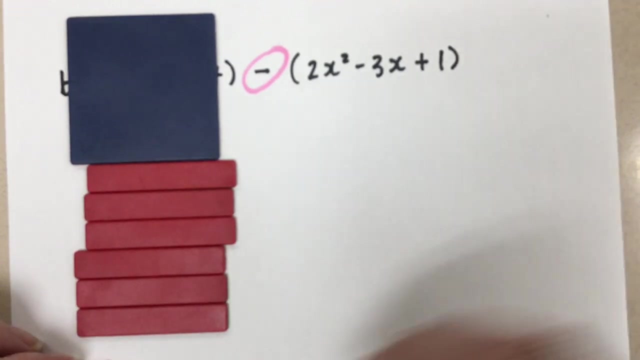 Three, four, five, six, Like this: Okay, And what was it Minus four? Oh boy, we're going to maybe run out of space here. One, two, three, four, Okay, Now we're going to get this polynomial. 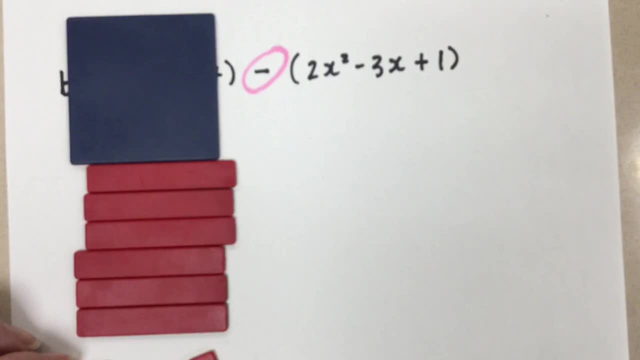 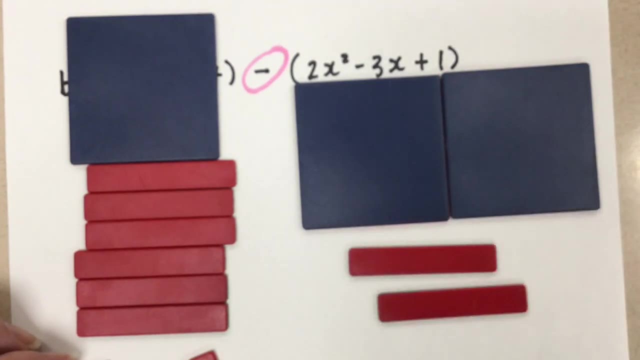 Let's ignore that minus in between. for now. Let's get this polynomial, So that's two x squared minus three x And then plus one. So this is now how we're going to approach the subtracting in between the two polynomials. 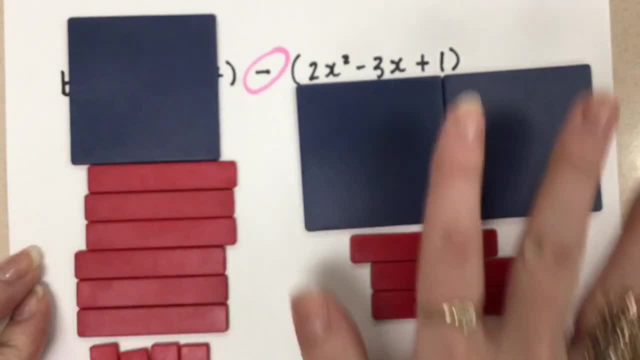 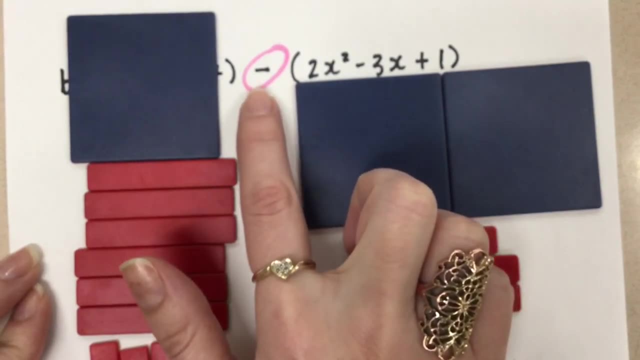 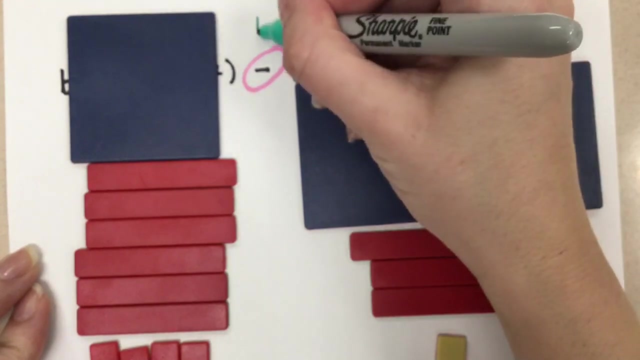 In the previous question we added them together. So we just combine these two together and that's it. But when it's subtracting, subtracting is actually adding the opposite of this whole polynomial. So if we think of this as adding the opposite of this, 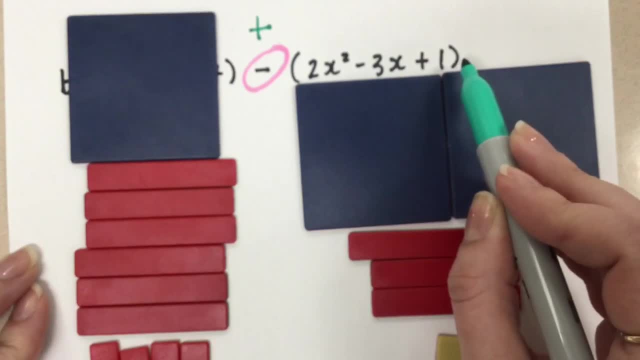 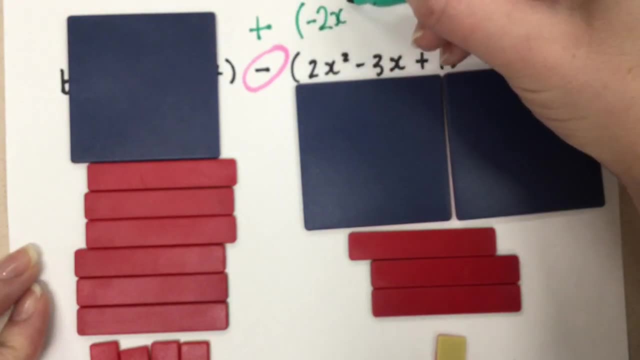 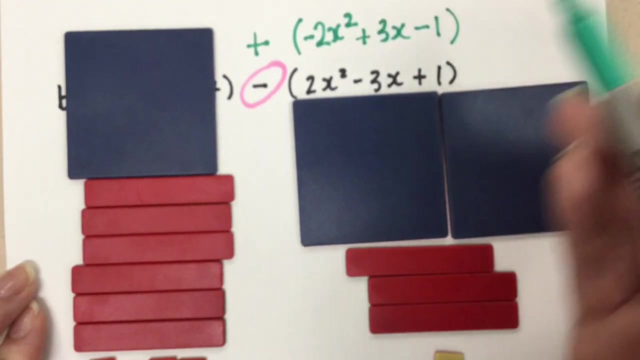 the opposite of a number or a term means change the sign. So instead in here we would have negative two x squared and then positive three x and then minus one. So if we interpret the question like this instead of how it was originally written, 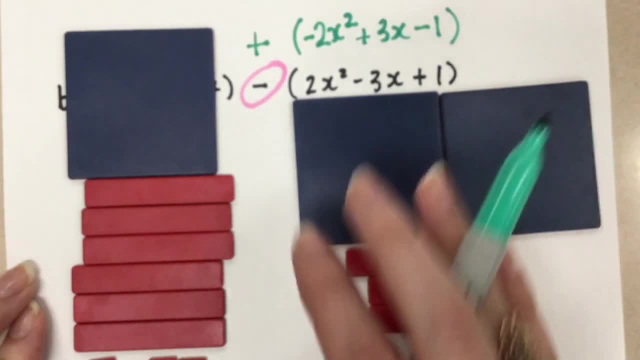 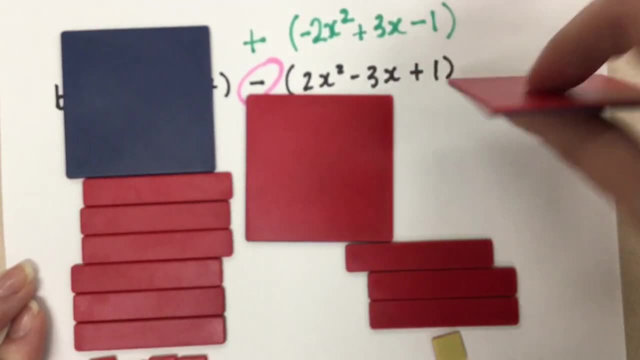 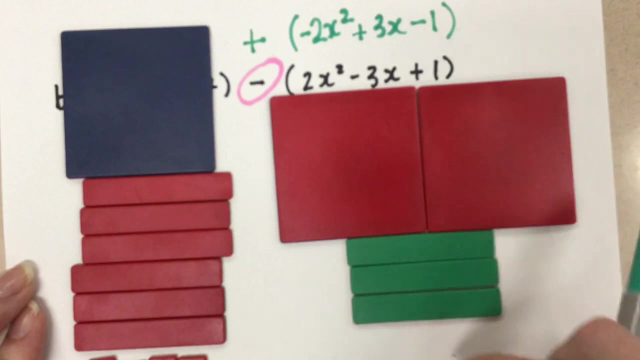 then we can just combine all the tiles together. So how do we change what we have here in the algebra tiles? Well, if we flip everything over, we now have the opposite. So now we have negative two x squared, and now we have positive three x and now we have negative one. 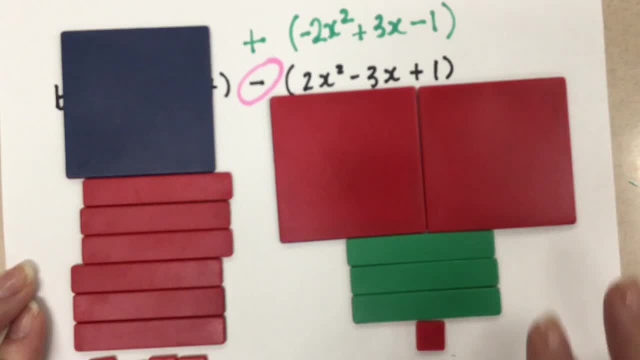 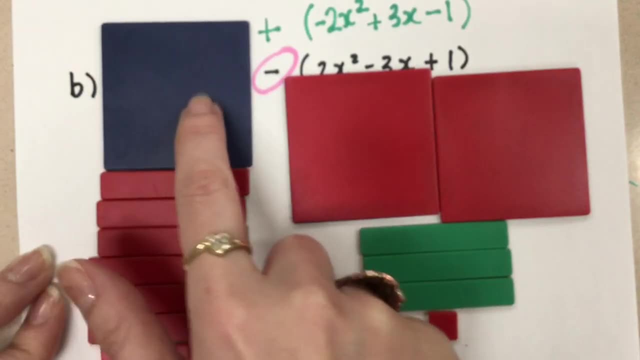 And at this point- this is like the previous question we did- We can combine all of these tiles together. Let's do that In the first term. here we have a positive x squared and negative two x squared, So when we add these together, that creates a zero pair. 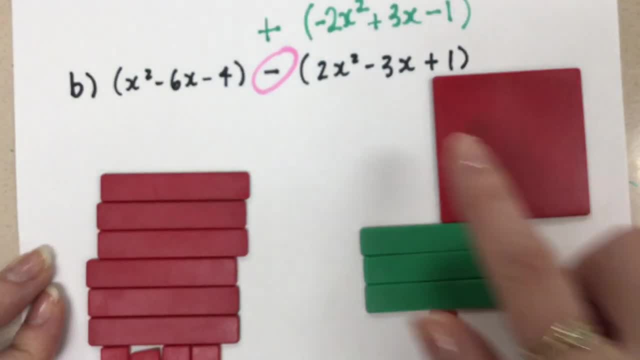 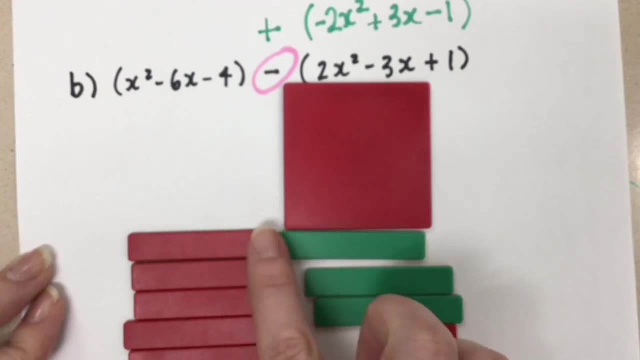 We're going to get rid of that tile and we're just left with this one. With our x's, we do the same thing. There's a zero pair, Let's get rid of it. Here's another zero pair: Get rid of it.